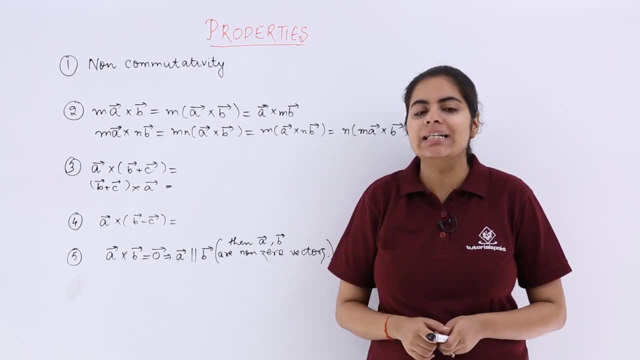 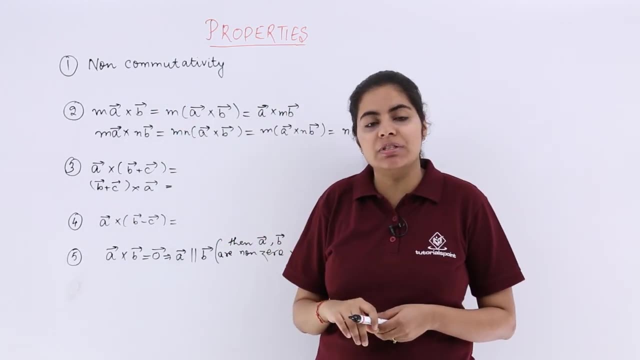 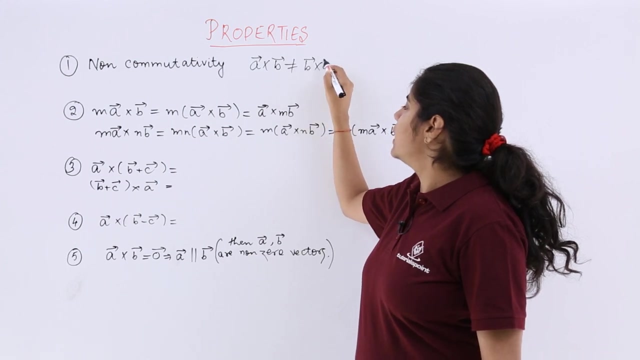 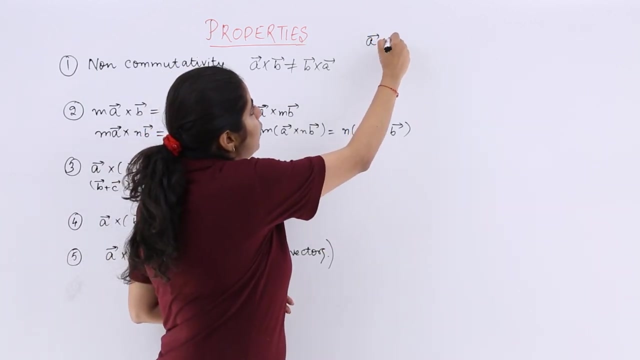 Remember once we studied the properties of dot product. This time is to study the properties of cross product or vector product. So the first property is non-commutativity. That means definitely your A cross B is not equal to B cross A. This is non-commutativity in case of vector product. Why? Because if I have to speak about A cross B, that will be A, B, C. 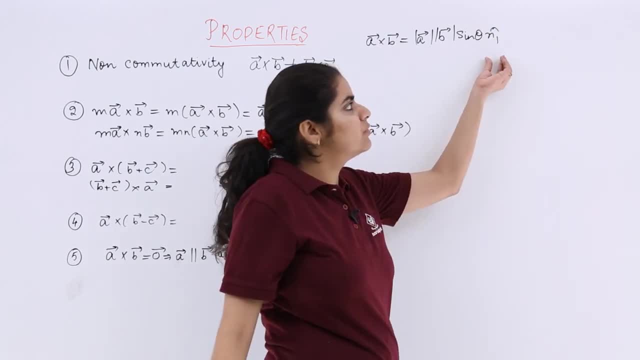 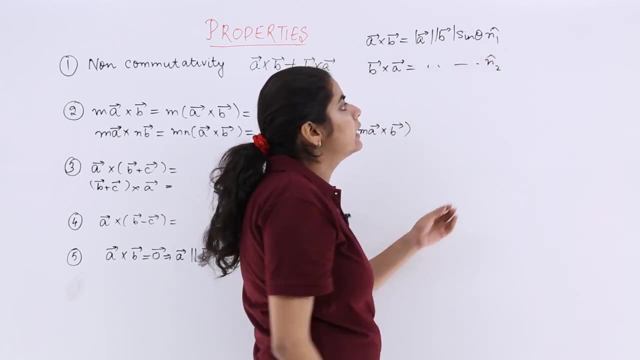 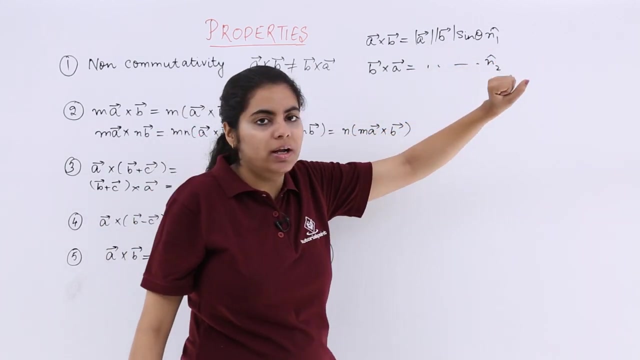 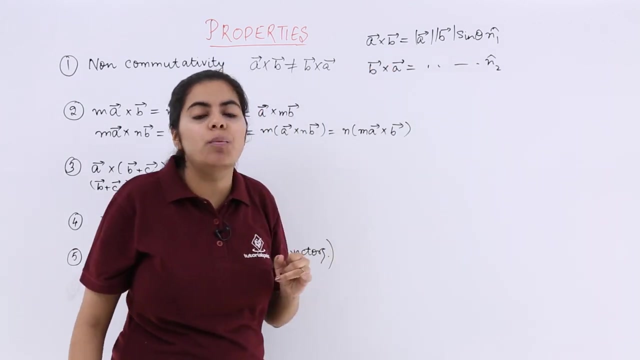 Sin theta n1 cap, a unit vector. And in the second case of B cross A, things will change to another unit vector n2 cap. So in the first case your vector A, B and n1 unit vector will form a right handed system. But here B, A and n2 will form a right handed system. So the order changes and hence the commutativity is not equal to B. 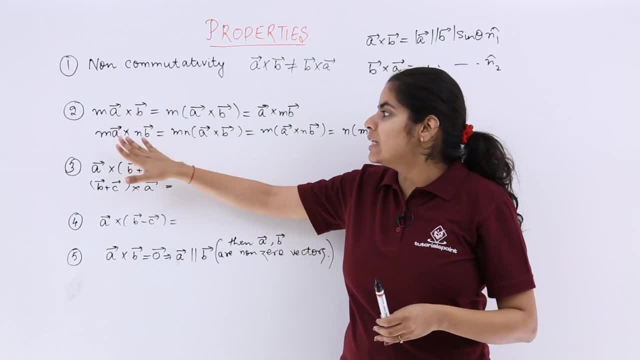 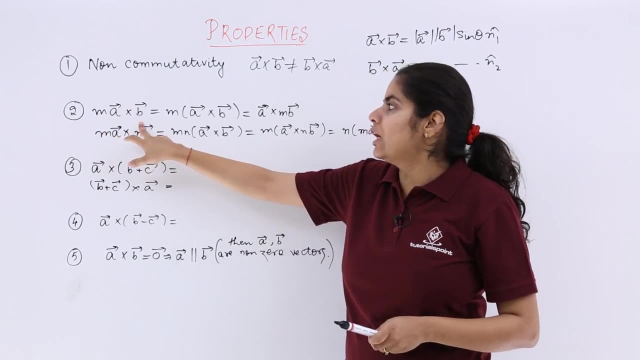 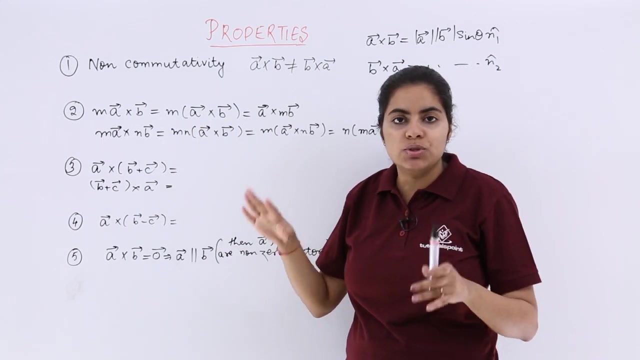 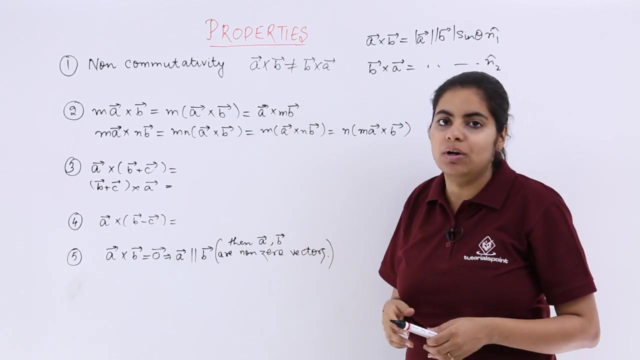 So it is non-commutative. The second is stating the properties when scalars are introduced. So M is a scalar. So M A cross B can also be solved. Like first you draw the system with A cross B, you solve it and then multiply the scalar. Or you can take M with B first and then cross product accordingly. So it is like that. But when two scalars are introduced, one is M, another is B. 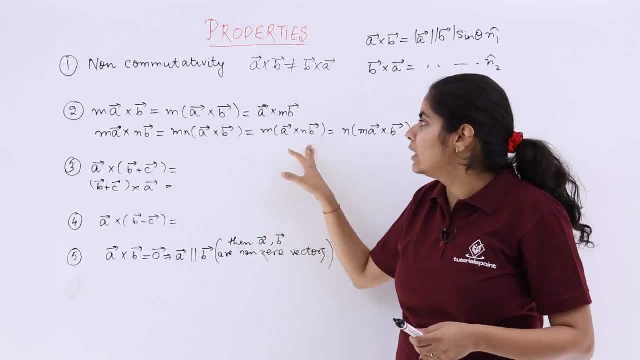 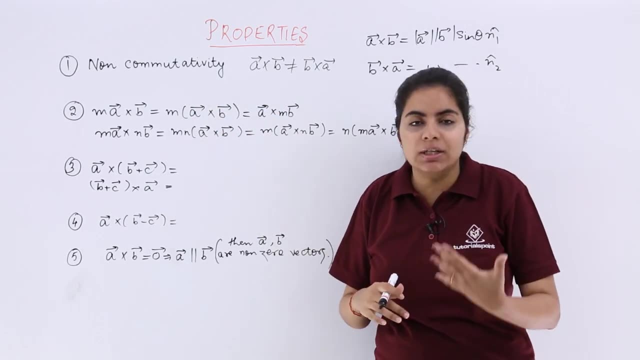 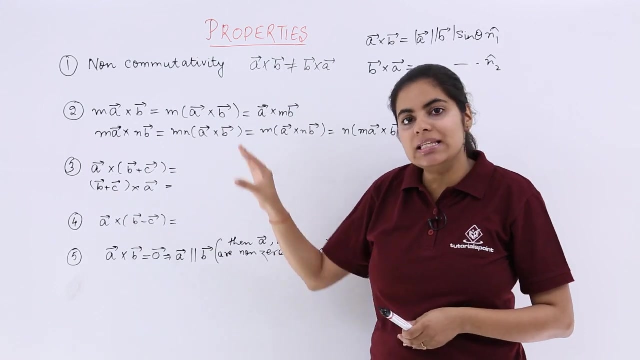 And another is N. Then what happens? Individually M and N can be separated. Then firstly M can be separated. N can be treated with B and so on. So this is just simplifying your calculation. Whatever suits you best, you can use it. So introduction of scalars in the case of vector product is this property all about. 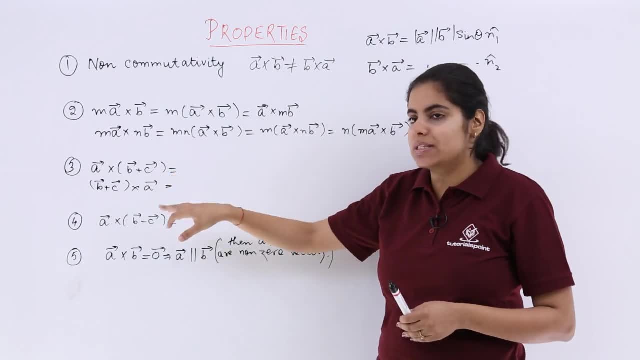 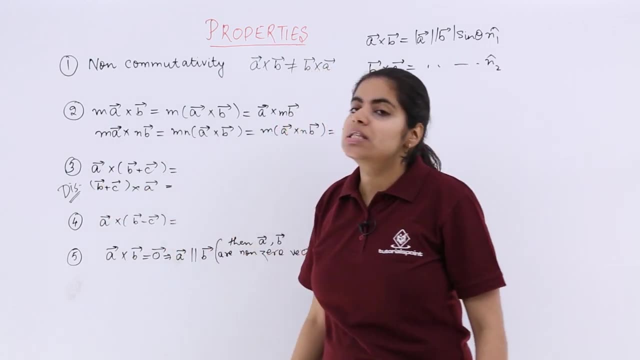 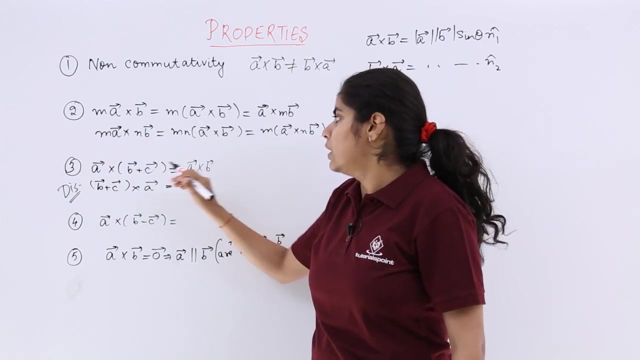 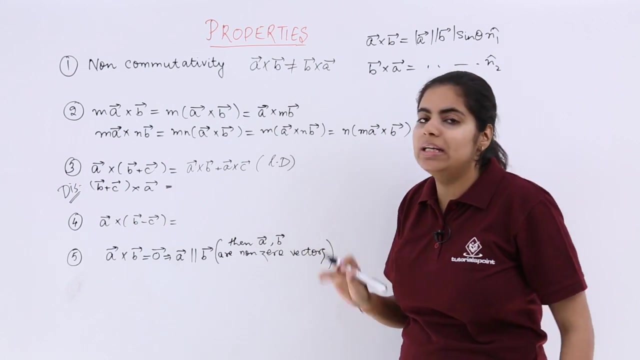 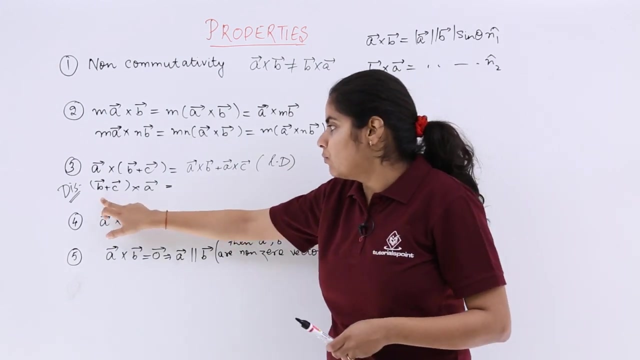 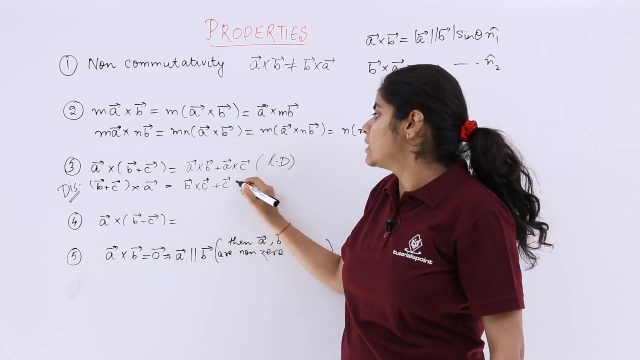 The third property as you can see. A cross B plus C. B plus C cross A. This is what you have done. So this is regarding distributivity. Distributivity is followed. Hence A cross B will be treated first. Then this is a plus symbol. Then A cross C. And this is known as your left distributivity. Hence I have written left distributivity means LD. I am sorry for that fumble. Now here B cross A. Introducing plus sign in between. Then is C cross A.